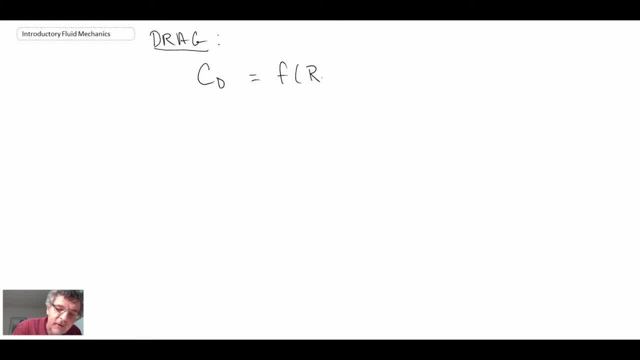 and the drag coefficient. we saw this in dimensional analysis earlier on in the course. quite often it will be a function of the Reynolds number, because things happen within the boundary layer around objects that have implications on the pressure distribution and that leads to impact on the drag coefficient, which we will see in this segment and the Reynolds number here. 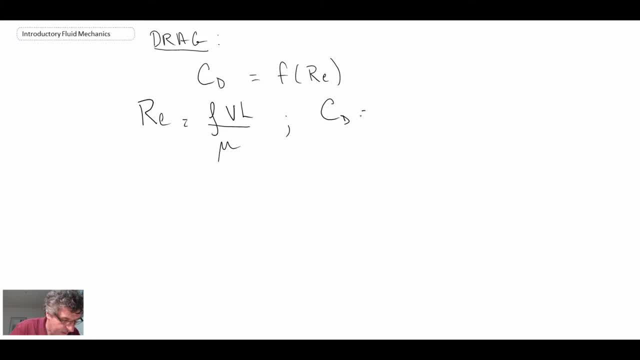 and the drag coefficient would be the drag force, whatever it might be, and we divide by the dynamic pressure and you'll notice in both the Reynolds number as well as in the drag coefficient we have a number of things. V is the free stream velocity, so that's pretty easy. 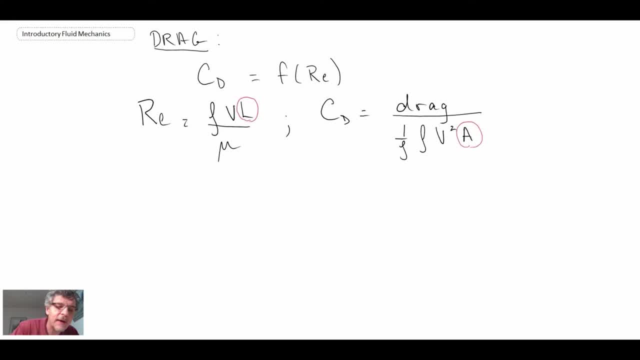 but we have this characteristic length and we have some area, and so you have to be a little careful with that, and so we're going to spend a little bit of time looking at how those are defined. so to begin with, the length in the Reynolds number. 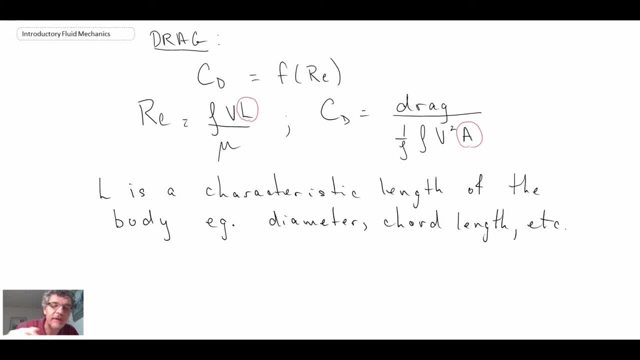 so it is some characteristic length of the body that is being investigated and it could be examples, could be the diameter, it could be the chord length if you're looking at an airfoil. the main thing is is, whenever you're using experimental data, 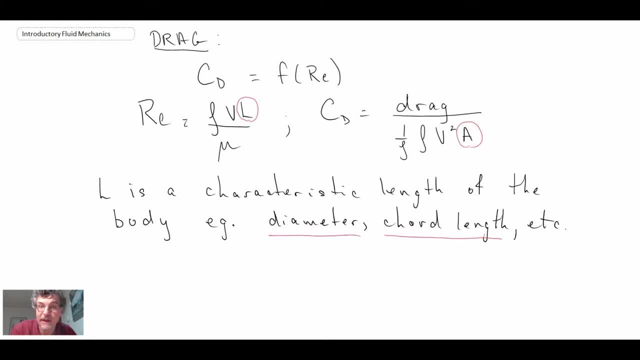 and drag coefficients. make sure you know what the characteristic length that they have been doing their experiments at or using the other thing is the area that is in the drag coefficient. so let's take a look at that so the area can be referred to as being the frontal area and that refers to the area as. 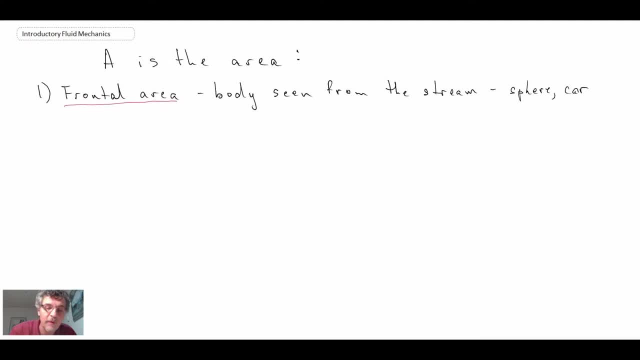 seen from somebody in the fluid moving towards whatever body you're characterizing, so that could be, as examples, a sphere or a car. it's basically the projected area as seen from somebody coming towards the body. so another form of area is the planform area, and that refers to the body as seen from above. 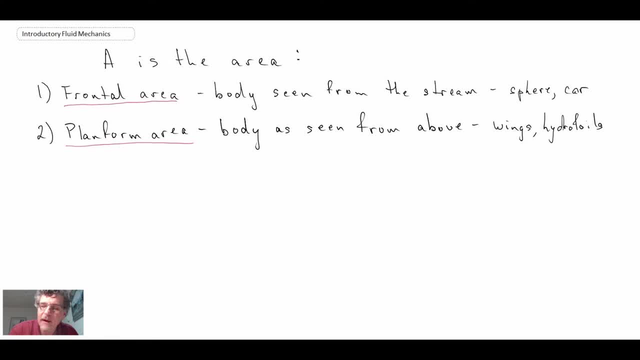 and so examples where you may use the planform area could be a wing. you might use the planform area, so the area, as looking down on the wing, a nautical application would be hydrofoils, and so looking at the area from the top of a hydrofoil, so that's planform area. 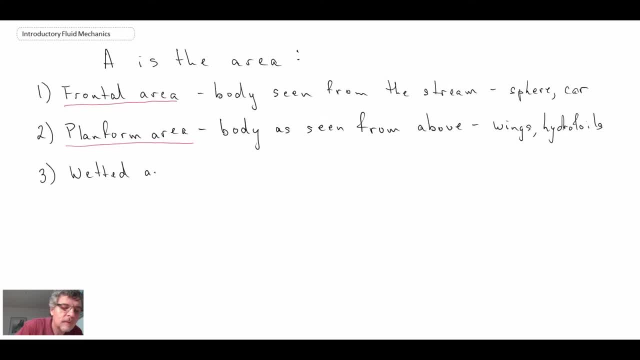 it's another area that could sometimes be used, and a final area that could be used is wetted area, and again that would be from a nautical application. so for ships or barges it would essentially refer to the component or the area of the ship that is in contact with liquid. so the main point here is just to be careful. 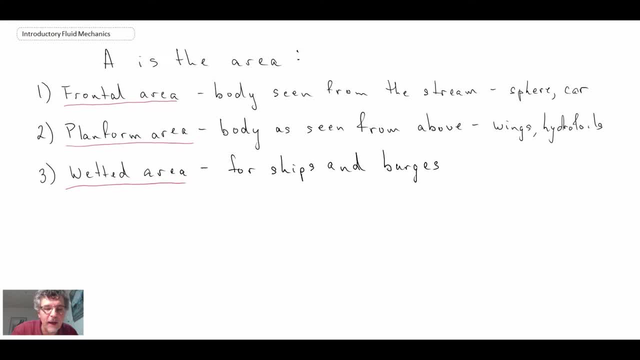 in terms of understanding what length or area has been used to produce the drag coefficient data that you might be using. okay, so that is the area and the length scale and the Reynolds number and the drag coefficient. now, when we look at drag drag on an object, for the most part, well, it consists of two main parts. 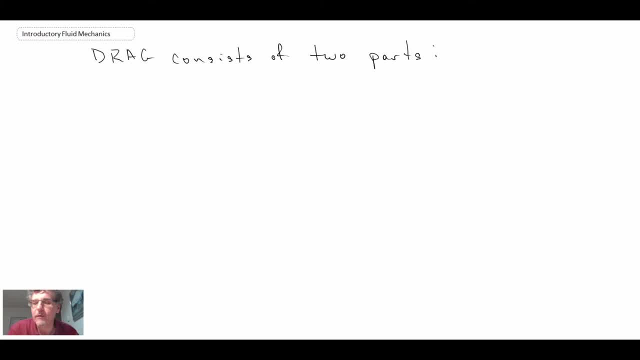 and we already talked about this earlier on in the last segment where we talked about the forces, we had shear force and pressure distribution acting on a body and that resulted in all of the forces- lift, drag, side force- and then the, the rolling moments that might be impacting the body. 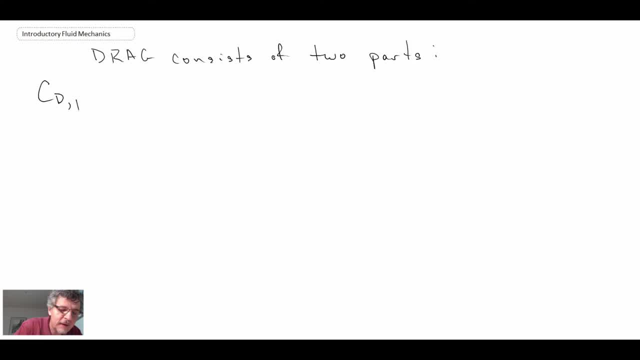 but when you look at drag, we have drag associated due to pressure, and this is sometimes called pressure drag or form drag, and what the pressure or form drag refers to is the low pressure zone that develops behind the body. what will happen we'll see in a moment. you get separation and there's low pressure in the 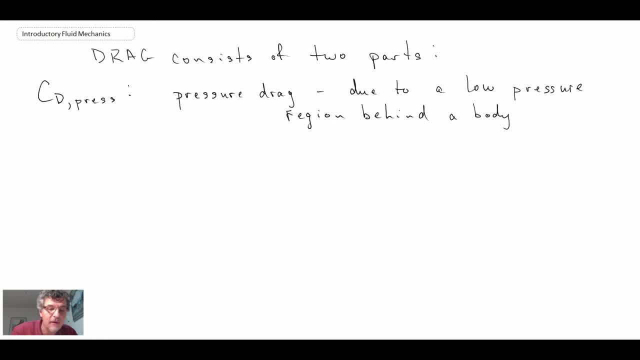 separated fluid zone and that leads to a force acting in the direction of the velocity, which is represented as a drag, and the other form of drag is attributed to skin friction or viscous shear along the wall, and this is referred to as being viscous try and we studied this rather extensively with the flat plate boundary layers we have looked at. 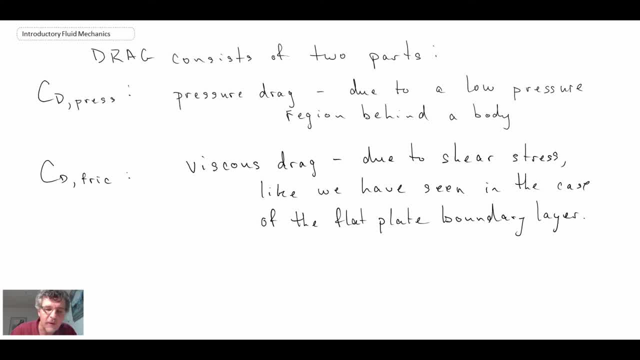 viscous drag has a wall, shear stress. so those are the two forms forces that can result in drag. we have viscous forces could be have form drag or pressure drag. so what we're going to do now, we're gonna take a look at a V video clip that illustrates some of these aspects and and so what we are going to be looking at here. 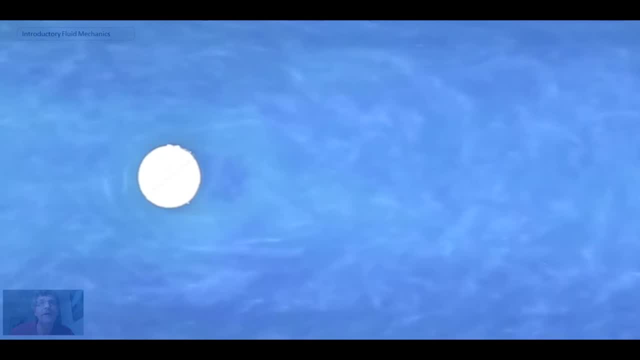 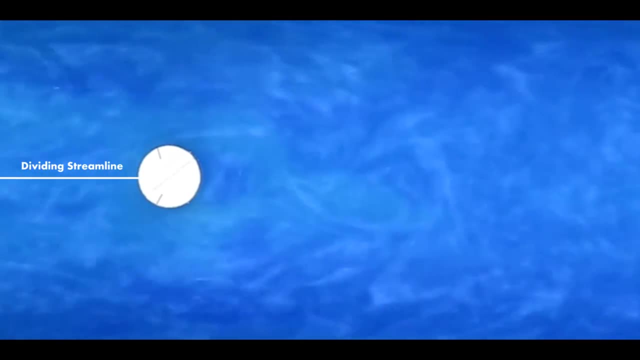 is the flow over a cylinder. and so here we can see flow over a cylinder and we begin. we have a dividing streamline on the upstream side and- and then I'm going to note a couple of points- that on the front of the cylinder those are separation points. so you'll notice the flow is separating at. 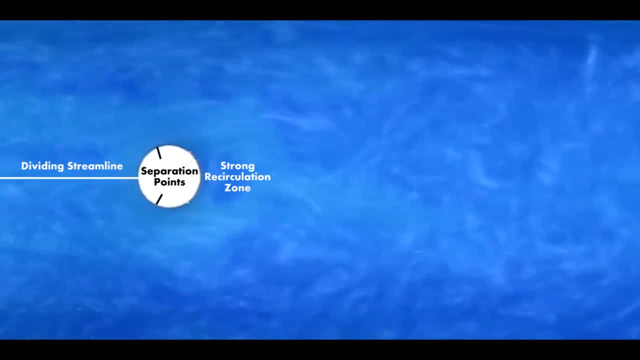 those locations, that's where the boundary layer is separating from the cylinder. downstream we get a strong recirculation zone that would have negative pressure or low pressure and that's what leads to the form drag. and then further downstream we have the von Karman vortex street. 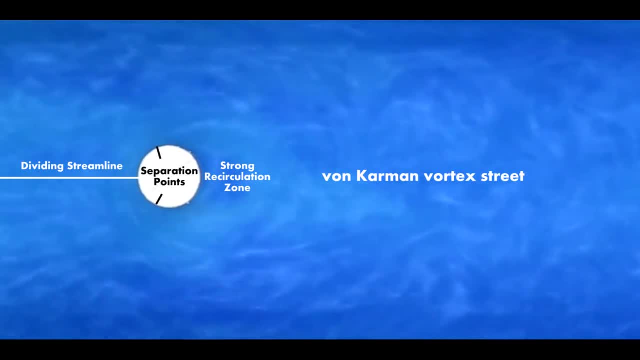 where there's a lot of oscillations and and that leads to different types of forcing and instability that can occur downstream. that's why, if you're traveling down the highway and you're behind a semi-trailer truck, you will find your car has side force going side to side and it's 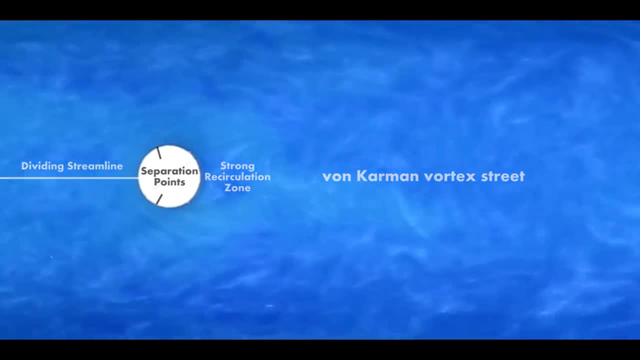 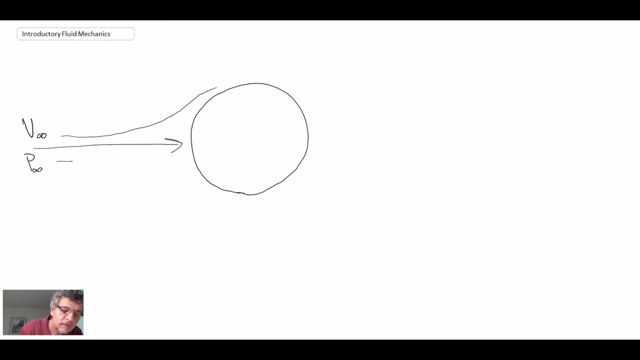 due to that vortex street behind the semi-trailer truck. so, looking at the flow of flow over a cylinder, let me just sketch it out and we'll denote some of the regions that we just saw. okay, so here we have a schematic showing what was happening within that cylinder. we come along, we have a leading edge or a front. 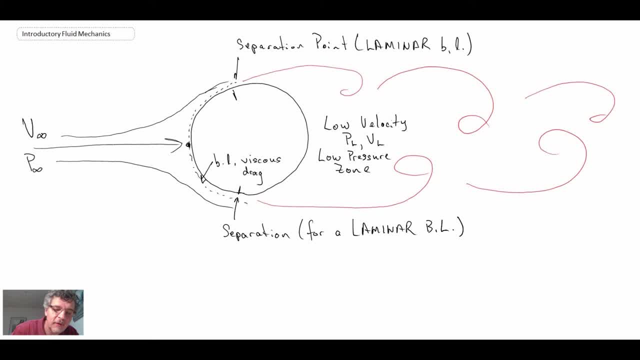 stagnation point, boundary layer forms and starts to grow as we go around the cylinder, either up or down, and then, once we get to a location, it's probably around 80 degrees, I think that's typically what is found. you get to the point where there's an adverse pressure gradient and 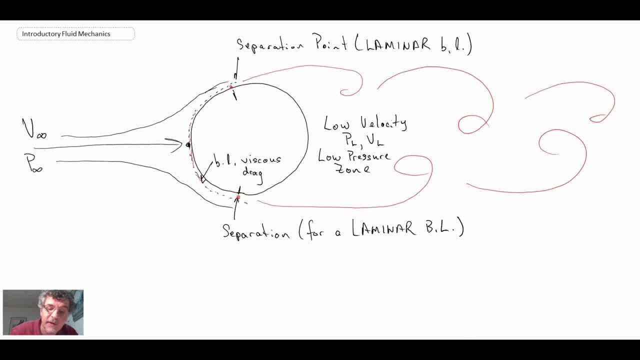 so the boundary layer lifts off, it separates. there's zero shear along the wall at that location, and when that happens, all of the vorticity that is in the boundary layer goes into this free shear layer that's forming, and and then you get these large scale structures that are downstream. 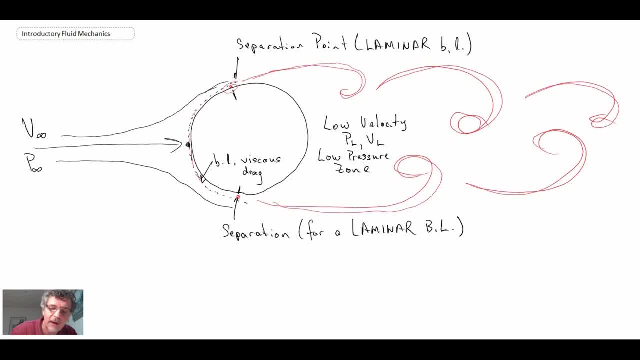 and that's what leads to the what we call the von carmen vortex street. now, where are the forces here? well, we have the boundary layer, viscous drag, so there is shear where the flow is attached, and so, consequently, we have shear force there, we have viscous drag, and then the other thing that's happening is we have a pressure distribution. 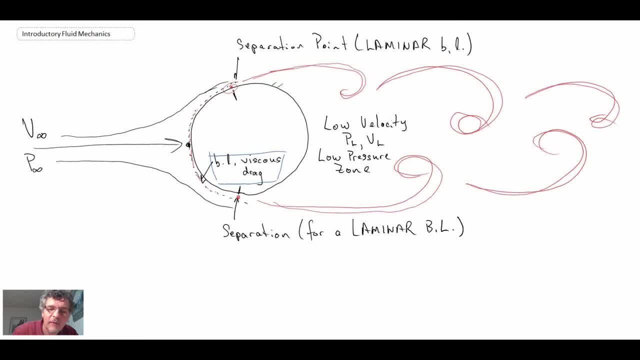 on the cylinder and in this region here, downstream of the separated flow region, we have very low pressure and that's due to the fact that we have separated flow. there's a strong recirculation zone there and that is one of the main contributors to the drag on a cylinder. 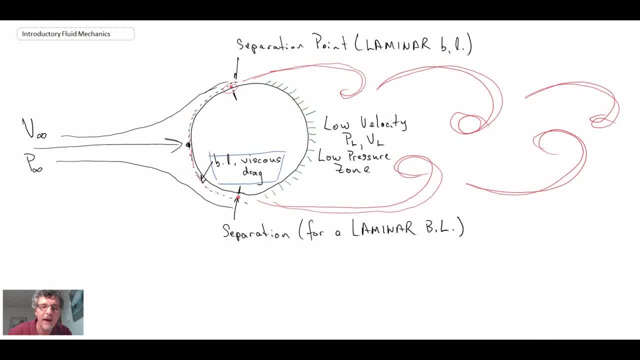 and and consequently those are the two forms of of drag that we're going to get into the cylinder- would be present in a cylinder or pretty much any bluff body where you get separated flow like you do with a cylinder. So if we were to try to analyze this and let's say we were to try to use the 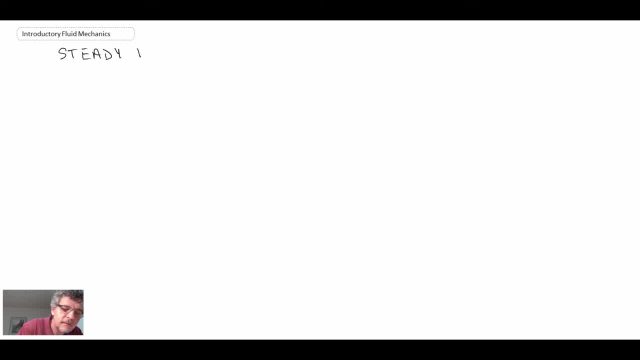 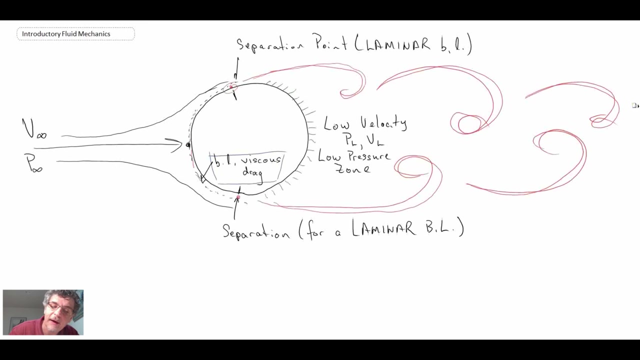 steady flow energy equation and we've seen the steady flow energy equation from our earlier analysis and I'm going to neglect the elevation term GZ- and if we were to try to do this between a point far upstream and let me go back, so if we were to try to apply this from this point here, 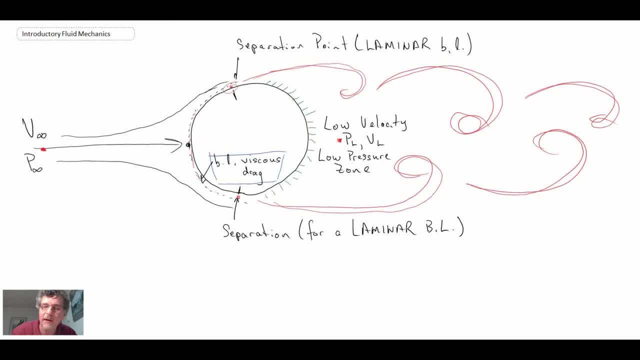 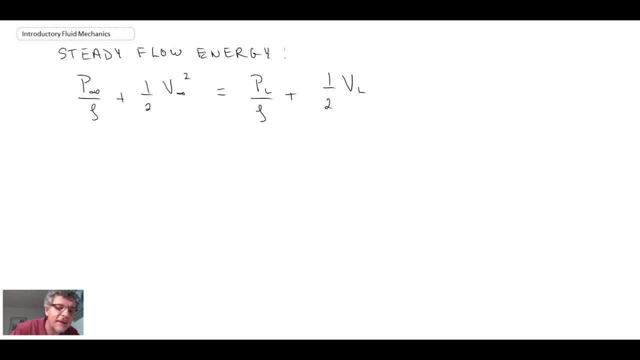 to, let's say, some point downstream in here, which would be where we have P low, V low. first of all, it would be very difficult to do, but the fact that the flow is not irrotational doesn't mean that this exists. We have to have something else on the right hand side. And what is? 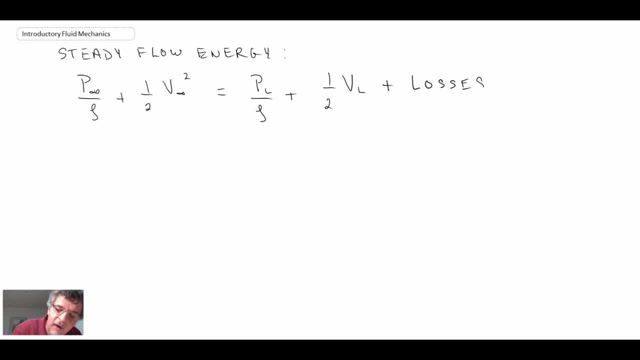 on the right hand side would be the loss term. So there would be losses associated with all of the turbulence downstream of the separated flow area And the losses we saw when we looked at pipe flow. we had the major losses for a pipe, or another way of thinking of this was: 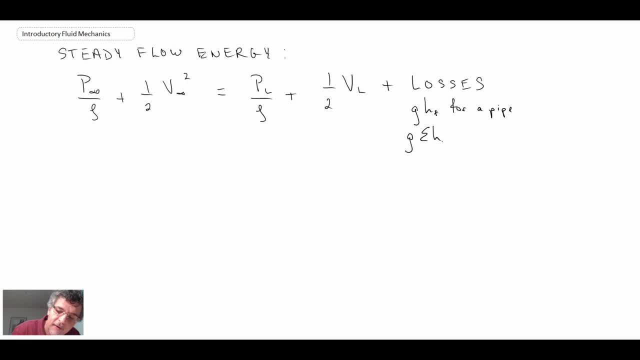 the when we were looking at the minor losses in pipe flow- things like elbows or expansions, so minor losses. So if you really wanted to apply this, what you would need to have is a way to be able to quantify all of the turbulence that is occurring in the. 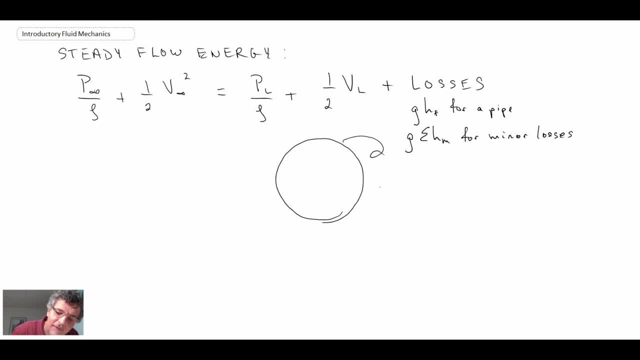 wake of the cylinders. So you would need to have a way of being able to account for all of the energy being lost in this area in order to be able to apply that. That's not a very good case. You probably would never apply the Bernoulli.